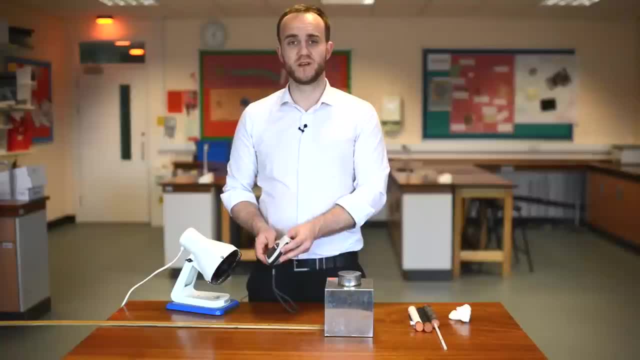 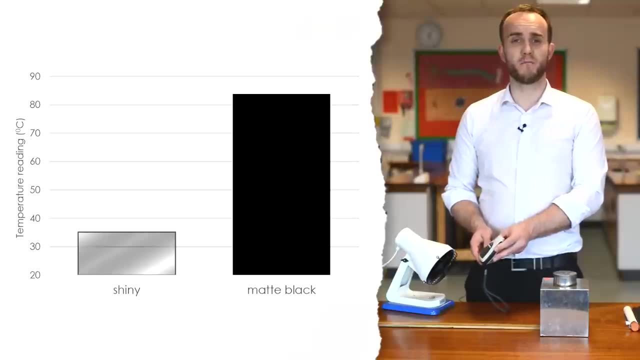 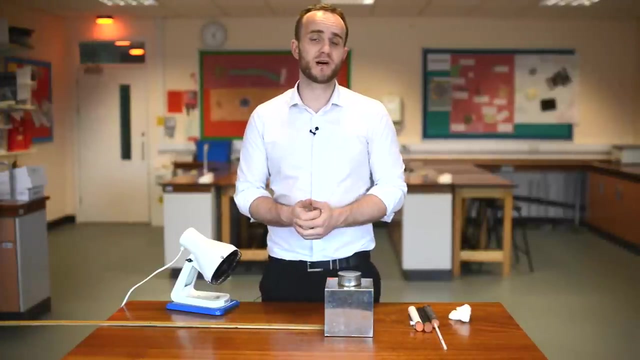 Wow, that's a really big difference. Now we have a temperature of 83.8 degrees celsius. That just goes to show that matte black surfaces are much better emitters of infrared than shiny surfaces. Now there are a couple of other experiments that you can do to test the absorption. 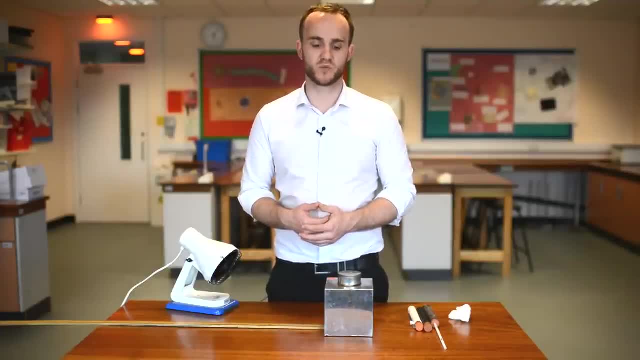 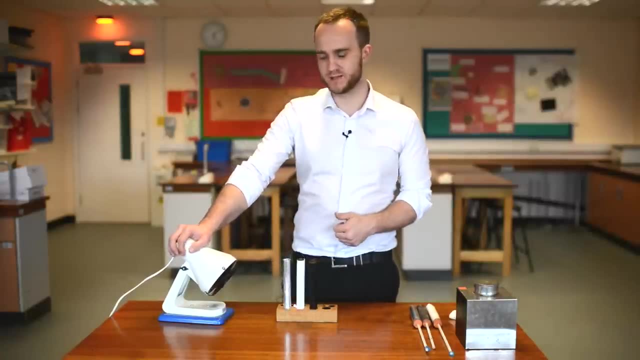 of different surfaces as well. Now, what I have here is an infrared lamp. Most bulbs give out infrared, but these kind of lamps give out more infrared. What I have here are copper tubes with a bung in one end, and they are covered in different materials. 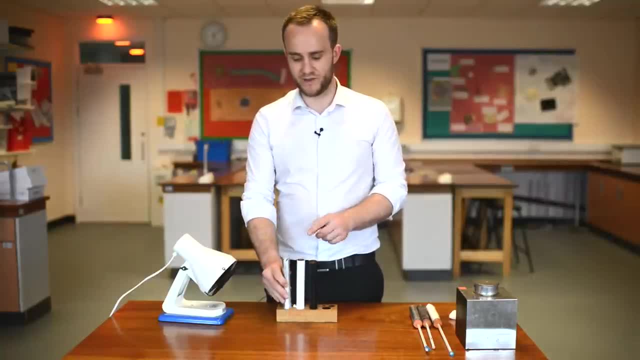 We have a shiny material. we have a matte white material and a matte black material. What we can do is measure the temperature inside the copper tubes when we expose them to the infrared lamp. Just be sure that when you put a thermometer or a temperature probe in the tubes, that you put some 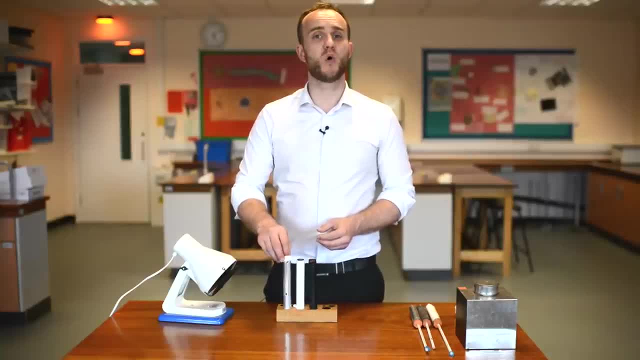 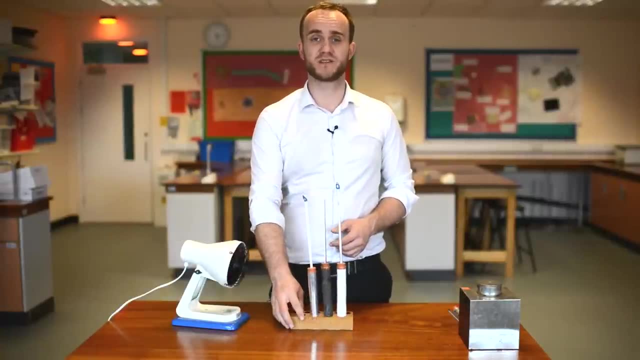 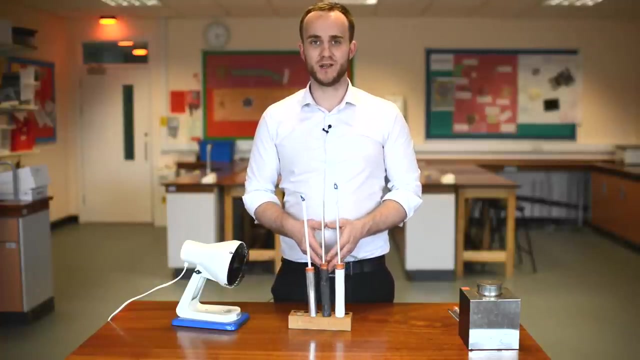 cotton wool around them because you don't want the thermometer to touch the sides. Another easy method is to use boiling tubes filled with tap water and they have different surfaces on them and a thermometer in a bung with the bulb in the water. As you can see, we have matte white, matte black and shiny surfaces If we expose them to infrared. 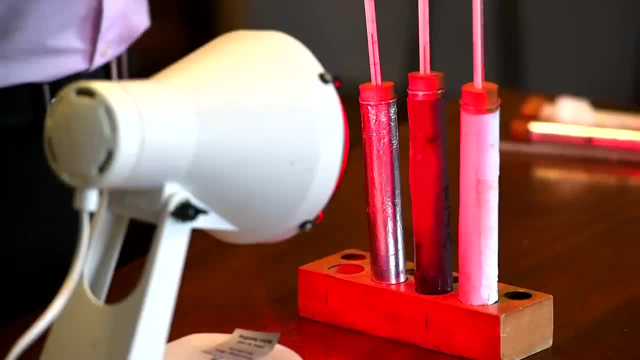 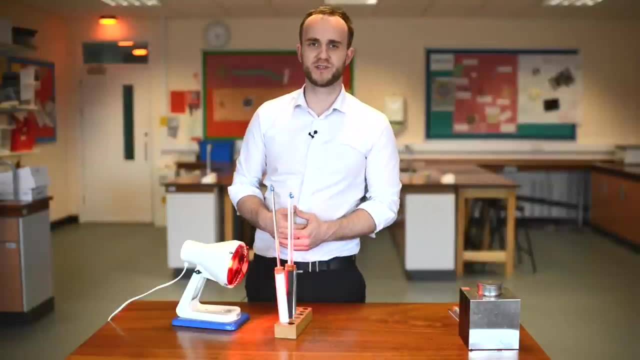 radiation, we'll see their temperature increase. What you can do is record the temperature every minute for 10 minutes, say, and see what happens, or you can just record their final temperatures after five or ten minutes and compare their temperatures. Now what you'll find is that matte. 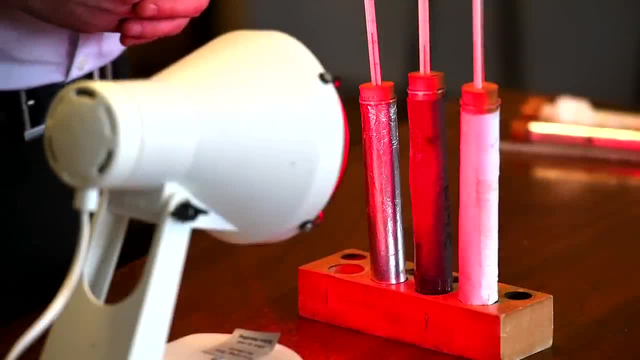 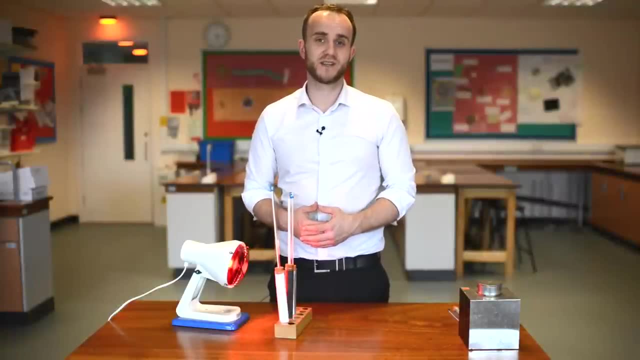 black is not only the best emitter of infrared radiation, it's also the best absorber, so it should have the highest temperature at the end. Shiny surfaces are not only poor emitters, but they're also poor absorbers, which is what you would expect, because they reflect light very well, and so they. 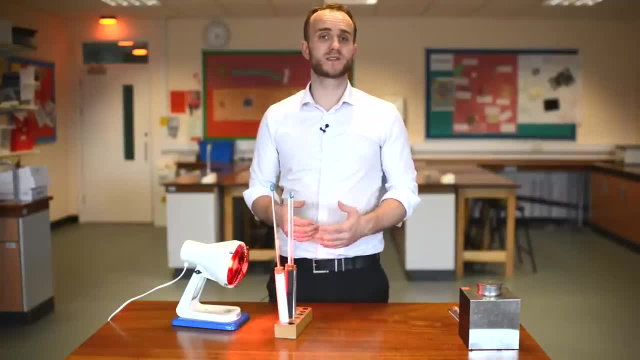 reflect infrared very well. also, Matte white is somewhere in between. it's not the best, it's not the worst at either absorbing or emitting. However, that's why, in a choice between a black t-shirt and a white t-shirt on a sunny day, it's the white t-shirt you want to go with, because if you wore, the black one, you'll absorb a lot more infrared radiation.